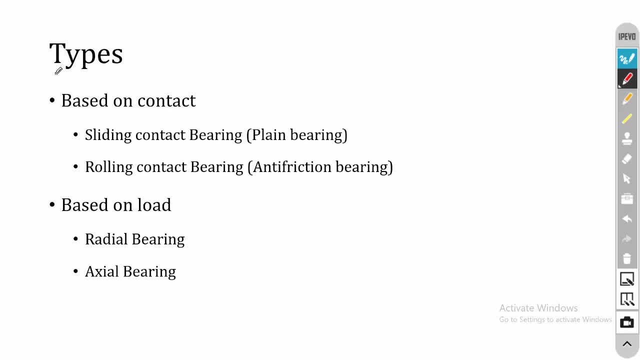 So the bearing is classified into two type in major. So one is based on contact. So based on contact it is splitted into two. One is sliding contact bearing and the other one is rolling contact bearing. So in sliding contact bearing the rotary part is directly fixed in the stable part. in rolling, 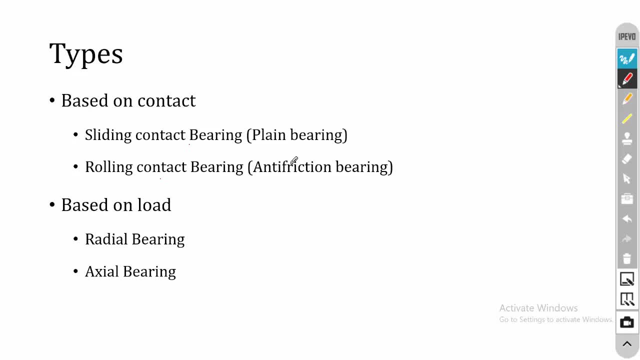 contact bearing. Some rollers or balls are used in between the rotary part and the stationary part. Then, based on load, it is further classified into two. One is radial bearing and the other one is axial bearing. So radial bearing is used to carry a high amount of radial load and the axial bearing 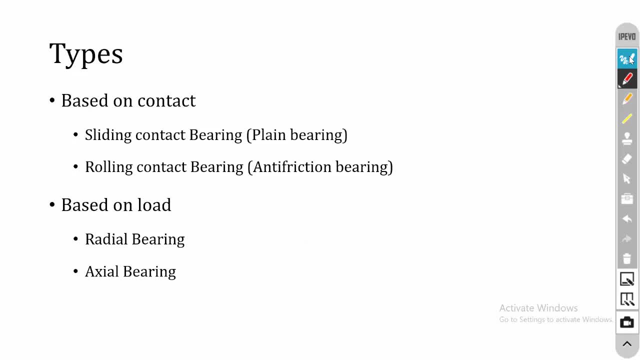 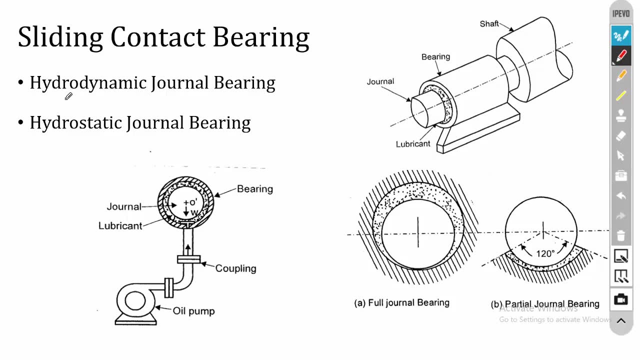 is used to carry a high amount of axial load. So we will see one by one. First we will start with the sliding contact bearing. So there are two types of sliding contact bearings. are there Sliding contact bearings? The first one is hydrodynamic bearing and the second one is hydrostatic bearing. 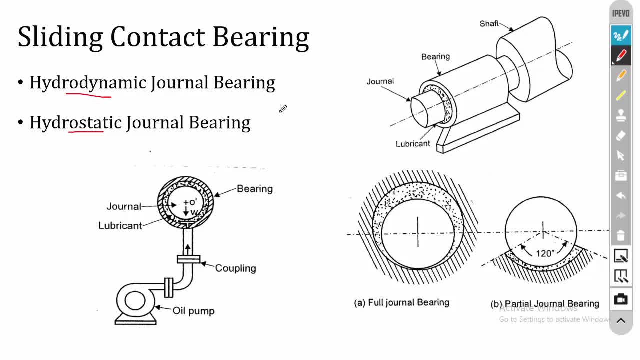 So remember that in sliding contact bearing we are not going to use any balls or rollers in between the stationary part and the rotary part, So we are going to use a lubricant in between the two parts. So look at this image. The shaft is our journal. 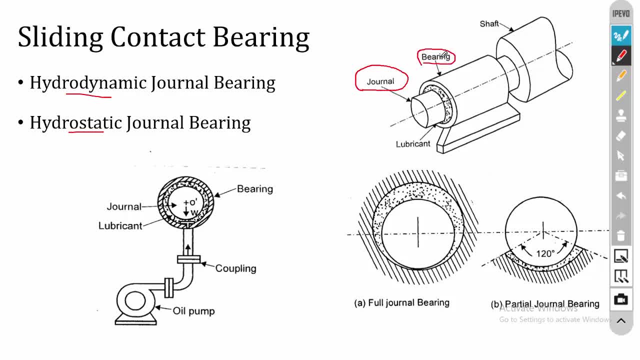 Then the outer part is our bearing. So the lubricant, Lubricant, is introduced in between the journal and the bearing to reduce the friction. So here there is no additional elements, are there? Only lubricant, like oil, grease or graphite are used to reduce the friction. 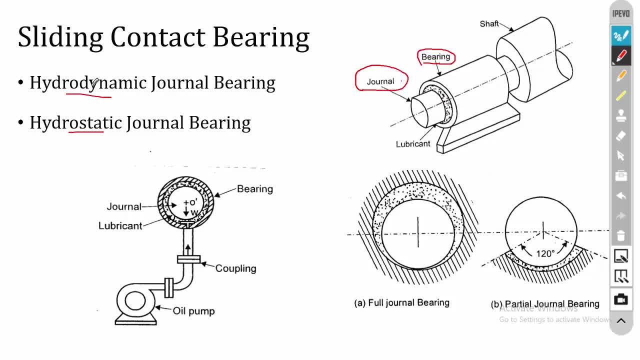 So this is about sliding contact bearing. Now coming to the hydrodynamic bearing. So in case of hydrodynamic bearing, we have a small amount of lubricant in between the journal and the bearing, So the lubricant is applied manually. So when the shaft starts to rotate, then this will be the position of the journal. 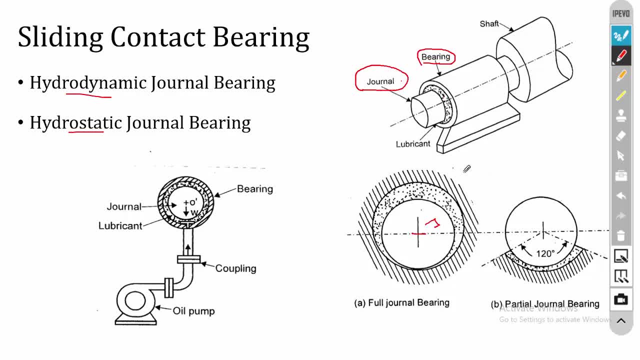 So at rest state. this will be the position, This is our journal and this is our bearing. And when it starts to rotate because of the centrifugal force, the journal will come to its center And you will have a hydrodynamic layer of lubricant throughout the bearing. 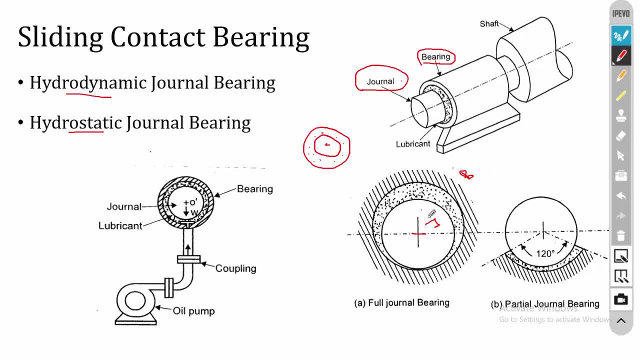 So this is the position of the journal, This is the bearing. So at rest state, the journal will be touching at the bottom edge. Then, once it starts to rotate because of the centrifugal force, the journal will come to its center point and a thin lubricant film is formed. 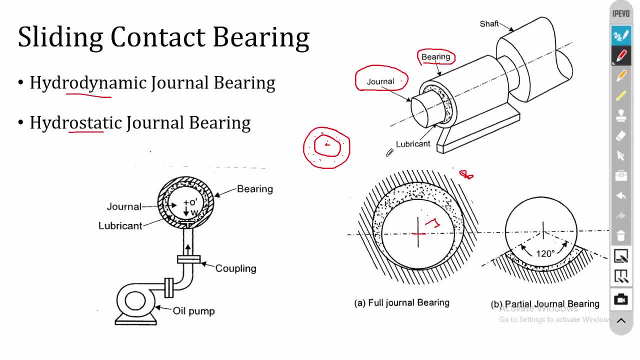 So in case of hydrodynamic bearing the lubricant is applied manually. There is no external pumping force is used for applying the lubricant. Then in the case of hydrostatic bearing, then oil pump is used, Because in hydrodynamic bearing we are applying the lubricant manually. this will be suitable. 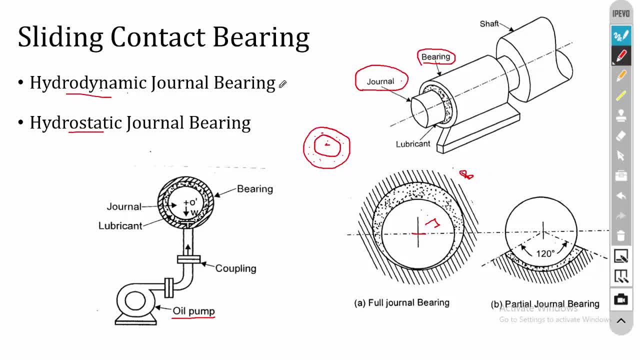 for medium and low load application. So in this case, if you go for high load application, then you have to go for hydrostatic bearing. in that case a oil pump is used to pressure the lubricant inside the bearing. So here the lubricant is pressurized and sent to the bearing. 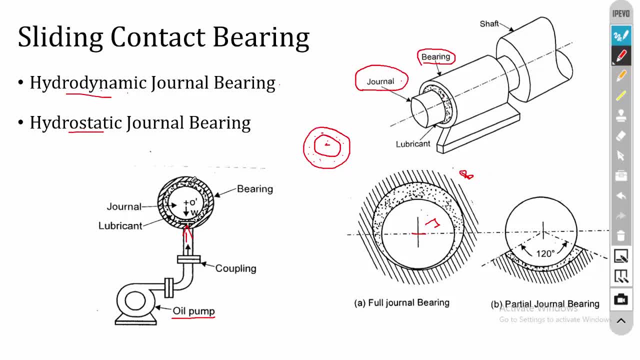 Ok, So o here. Because of this, in the pressurized liquid You will have a hidrostatic bearing, high amount of pressure of lubricant, and the pressurized lubricant is surrounding the channel. So that is the difference between hydrodynamic and hydrostatic channel bearing. 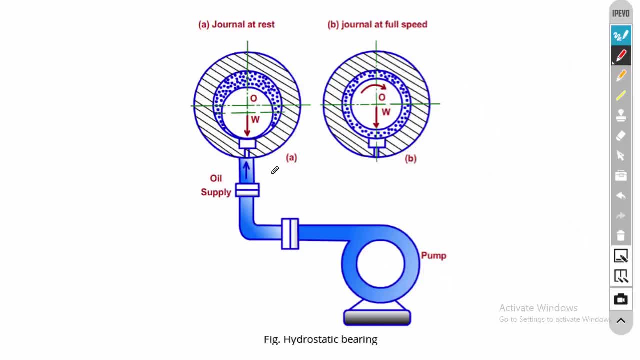 So you can see the image you will get a clear idea of. So this is the hydrostatic bearing. So at the initial stage the oil is pumped inside and when the shaft is at rest, then the shaft touches the or the channel touches the bearing. 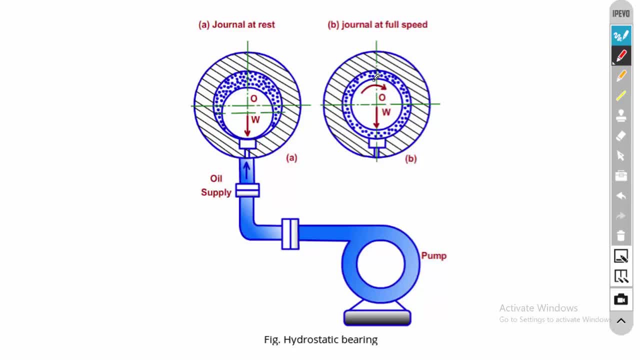 So here there will be a contact. So when the system starts to rotate, then because of the centrifugal force the channel will come to its central position and you will have the lubrication frame throughout the 360 degree. So in case of hydrodynamic bearing the lubricant is applied manually. 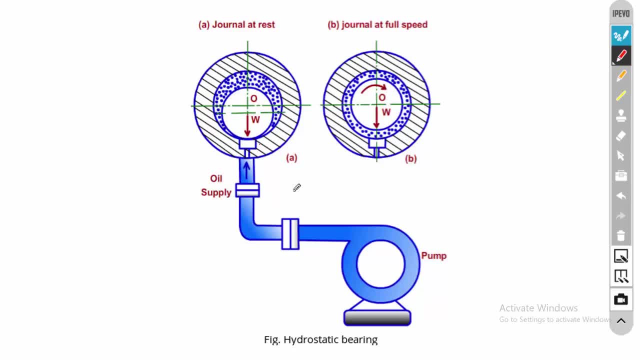 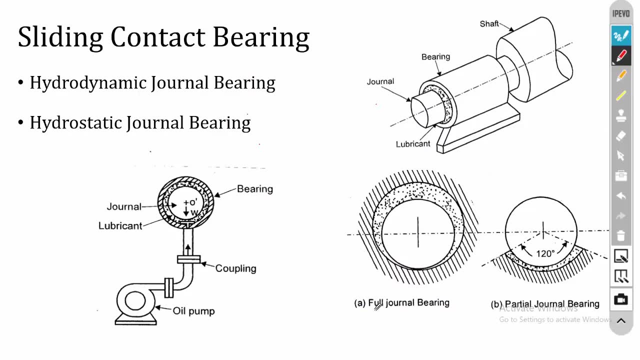 In case of hydrostatic bearing, the pump is used to pressurize the lubricant inside the channel. So there are two types of channels, are there? One is A full channel bearing. So in case of full channel bearing, we have 360 degree of bearing, that is, covering the 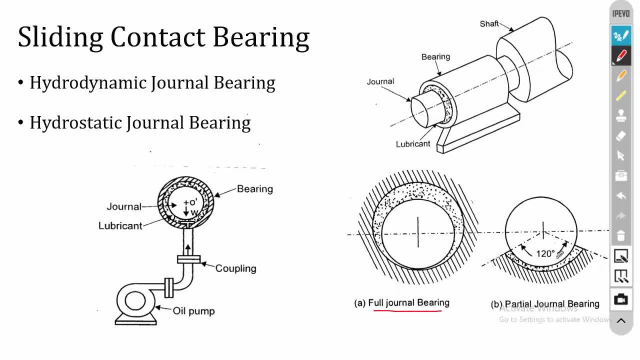 channel. In case of 120 degree channel bearing or partial channel bearing, then we have here it is 120 degree. we have 90 degree channel bearings, So here for the 120 degree alone the bearing is used. So we have channel for 360 degree and the bearing covers only the 120 degree. 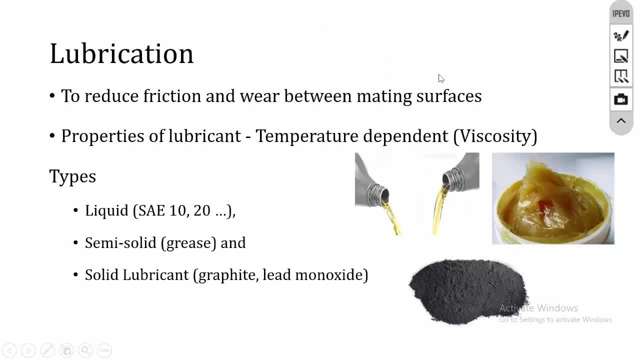 So the next type of bearing is, before that, the type of lubricant used in hydrodynamic as well as hydrostatic bearing. So the purpose for lubrication is to reduce the friction and wear between the mating surfaces and for selecting the lubricant for bearing applications, the viscosity is the important. 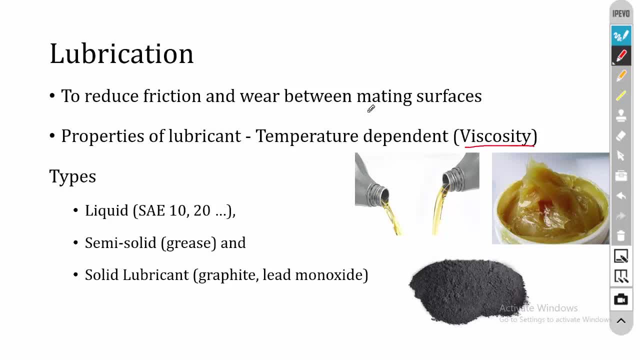 property, Because When the system rotates continuously then the temperature will increase And that means the lubricant will be coming down in the lubricant itself. So for lubrication increased and we know that when the temperature is increased the viscosity will come down. okay, 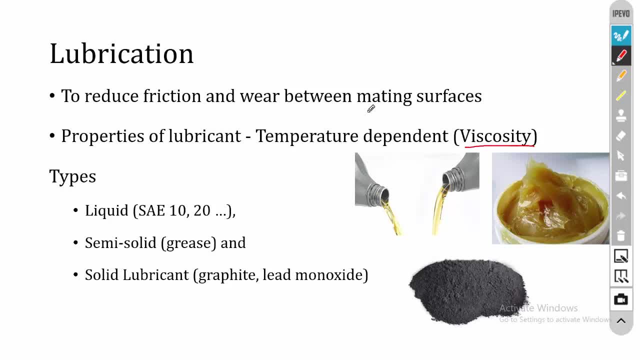 so we have to focus on the viscosity. then that is the important property for lubricant selection. okay, so in lubricant we can use liquid lubricant like sae 10 or sae 20 or otherwise. we can go for semi-solid lubricant like grease or otherwise. we can use solid lubricant like graphite and. 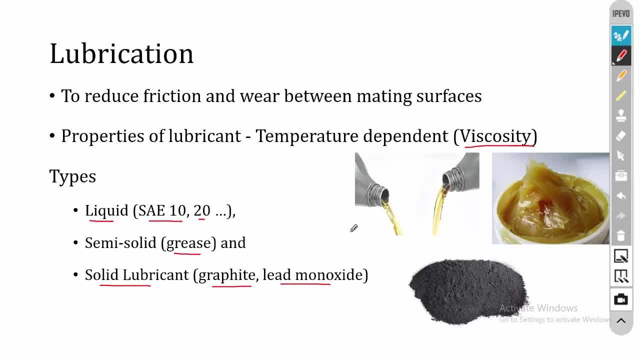 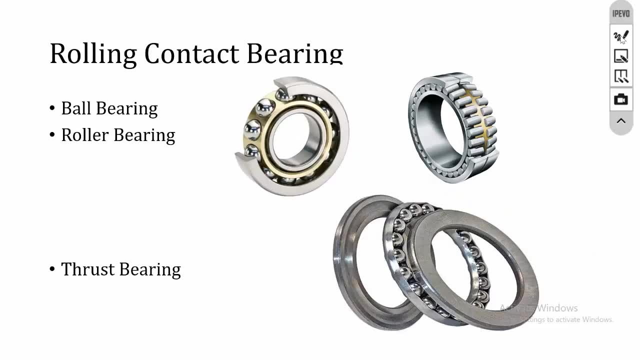 lead monoxide. okay, so any one of the lubricant we can use, based on our loading conditions. so the next type of bearing is rolling contact bearing. so in case of rolling contact bearing, the rollers or balls are used in between the static and the rotary part, so this is fixed to. 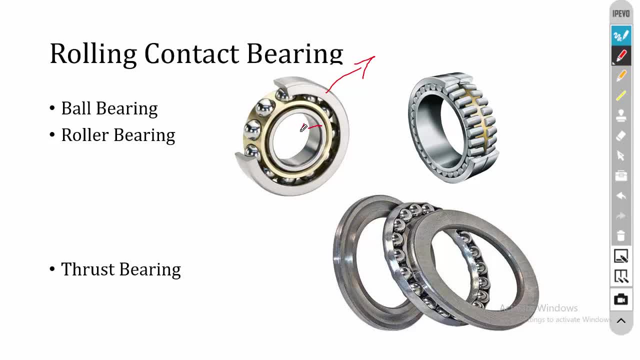 the support and this inside part is fixed to the shaft. okay, so the when the shaft will is rotating, the, the inside part will rotate and this rollers will rotate and it will not transmit the rotary or frictional force to the outer part. okay, so here the rollers and balls are kept in a cage for. 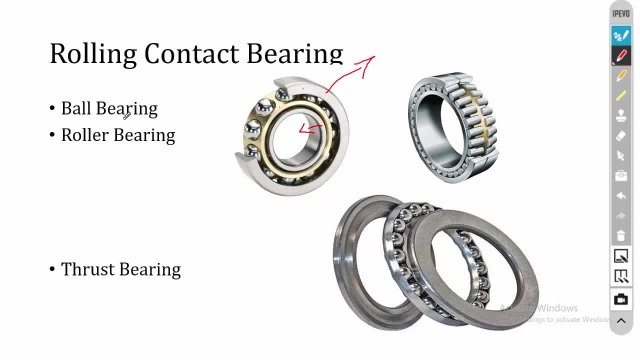 alignment. so there are three types of rolling contact bearings are there. the first one is ball bearing, so in that the spherical balls are used. then the second one is roller bearing, so here you can see that. so the cylindrical rollers are used in between the outer cage and inner race, then in thrust bearing. 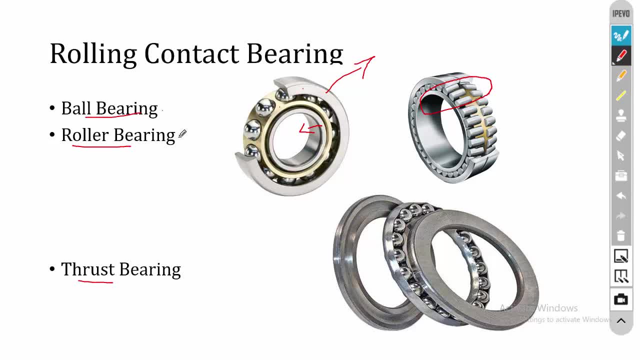 so thrust bearing in thrust bearing also, they are going to use balls and rollers only, but this thrust bearing will be will resist high amount of thrust loads. okay, so that is the difference between ball roller and thrust bearing. okay, so the outer race part is called as outer race, the inside 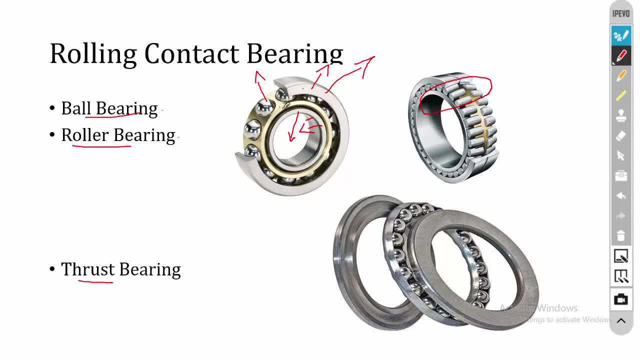 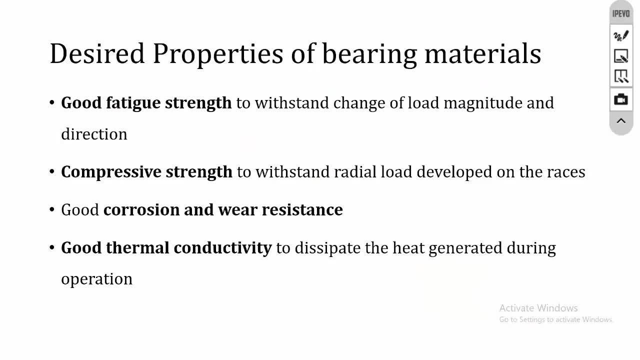 part is called as inner rays. then we have balls and we have gauze. okay, so these are all the four components of rolling contact bearing, so the desired properties of bearing materials. so first, the bearing material should have a high fatigue strength, because in shafts we may have some fatigue loads or fluctuating loads, so when the magnitude increases, then 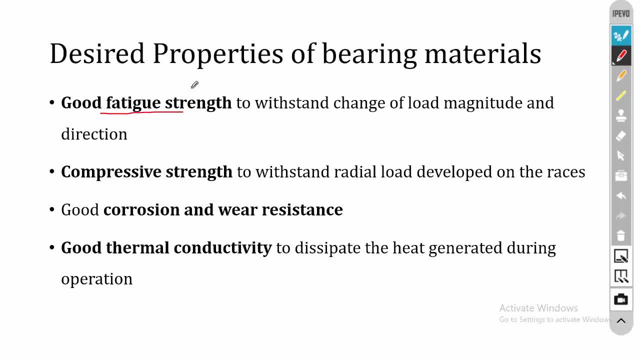 the bearing material should have the capability to resist the fatigue strength. then the second one is it should have good compressive strength, because when the radial load increases then high amount of compressive load is applied on the bearing. so the bearing material should capable of resisting the compressive strength. then the third one is good corrosion and wear. 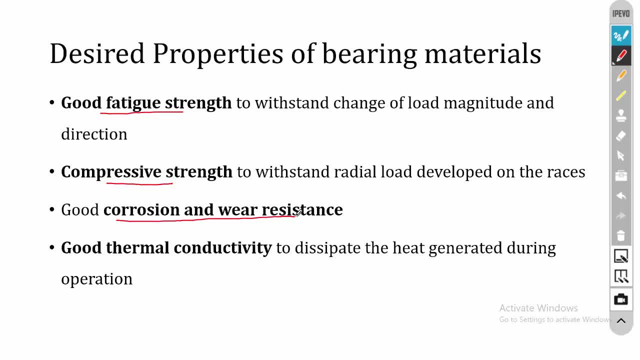 resistance. okay. so when the bearing is used for some flue gasses and so on, fluid carrying application, then the bearing material should have high corrosion resistance as well as the wear resistance. so the last and most important property is the material should have good thermal conductivity, because high amount of heat is generated in the bearing. 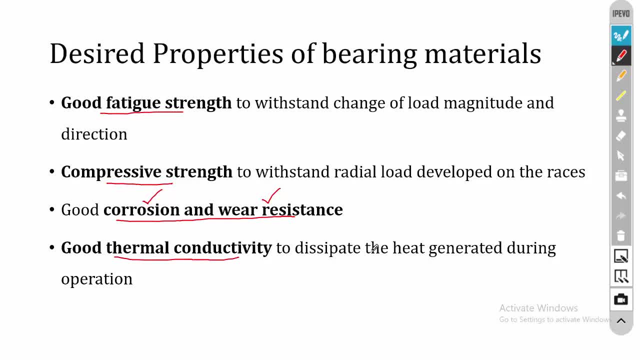 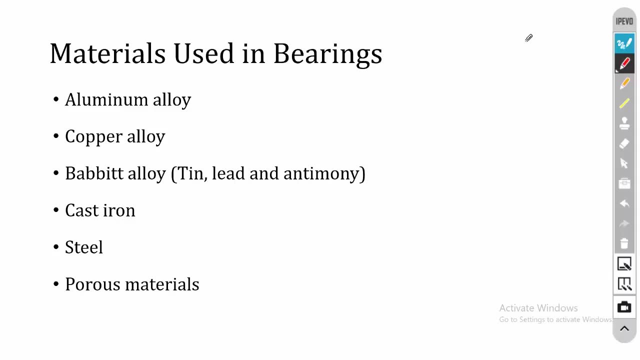 during continuous operations. so in that case the bearing should have a good thermal conductivity to dissipate the heat from the inside to outside. so these are all the materials used in bearings: aluminum alloys, copper alloys, then babbit alloys, then cast iron, steel and porous. so most of the medium load application bearings are manufactured.